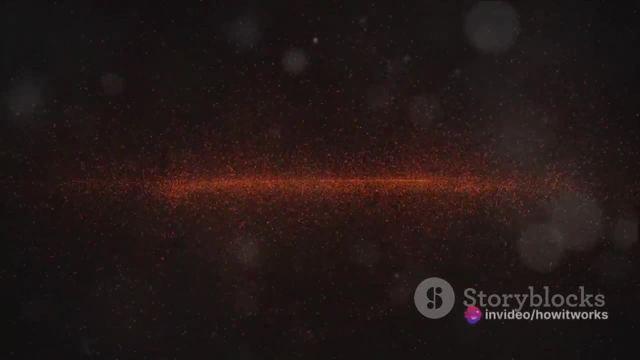 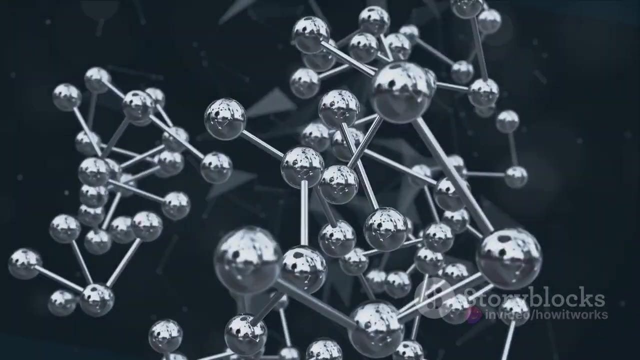 stable, with a lifespan that exceeds the age of the universe. But what if protons aren't immortal? What if they decay? The concept of proton decay is a fascinating hypothesis in the field of particle physics. It suggests that protons, given enough time, will eventually 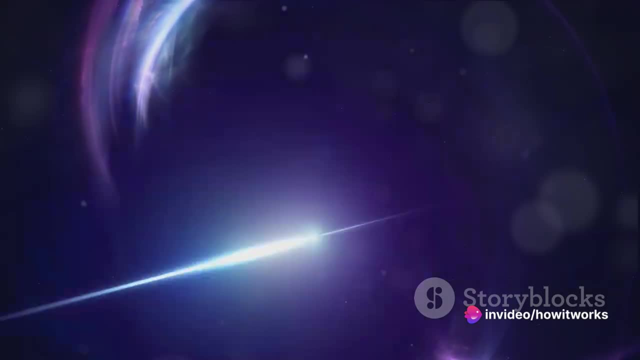 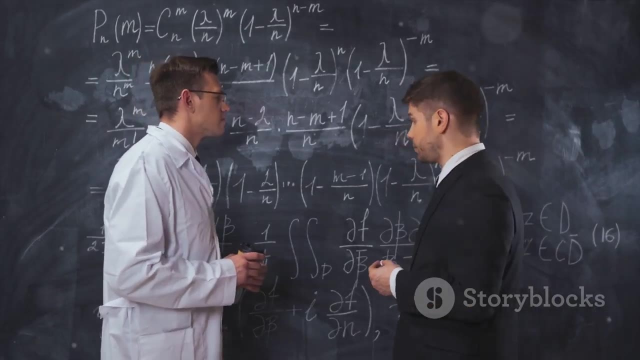 break down into smaller particles. This idea, though yet to be confirmed, challenges our understanding of the universe and the nature of matter itself. The question of proton decay also serves as a gateway into the realm of advanced theoretical physics. It leads us to explore: 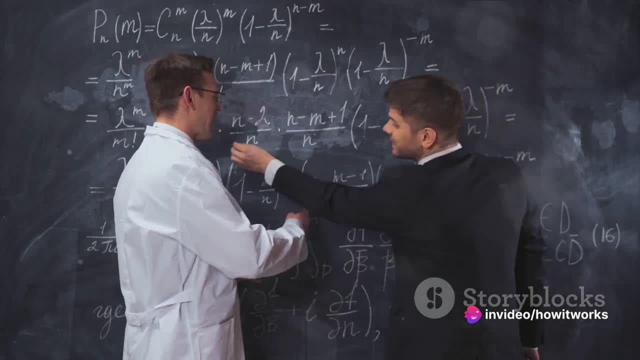 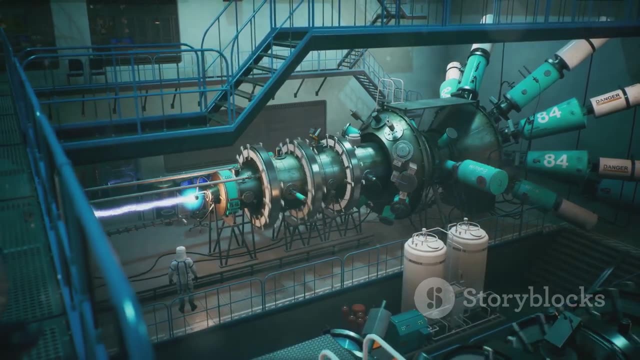 grand unified theories, or GUTs, and the concept of supersymmetry. These theories, while complex, offer a potential explanation for the decay of protons and other unexplained phenomena in the universe. So are you ready to unravel the mystery of proton decay? 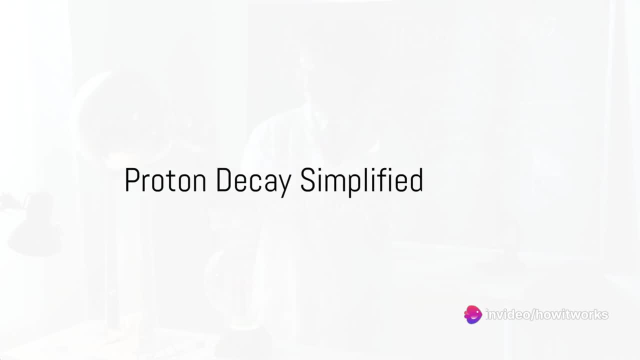 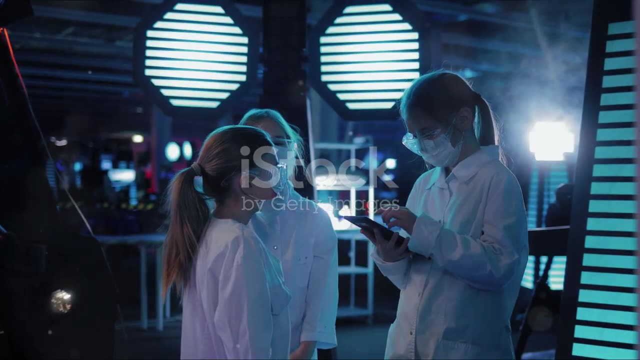 Let's dive right in. Imagine a proton, one of the building blocks of matter, as an apple that now never rots. Now that's a peculiar thought, isn't it? How can something as simple as an apple, a fruit that we all know and love, relate to something as complex as a proton? 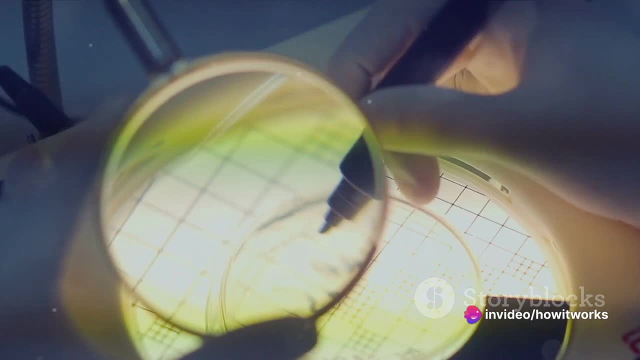 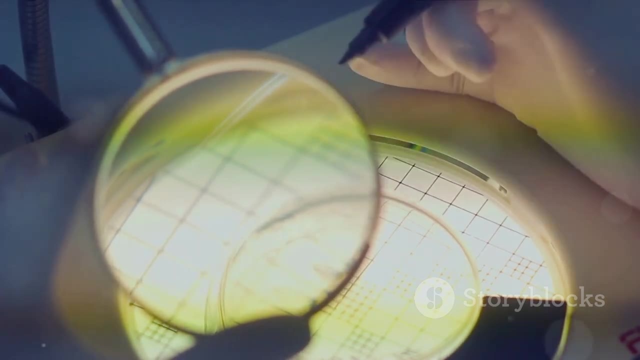 Well, let's dive in and find out. You see, just like an apple, a proton is a fundamental part of our world. It's one of the key ingredients that make up the matter around us, from the chair you're sitting on to the water you drink, and, yes, even to the apples you eat. But unlike an, 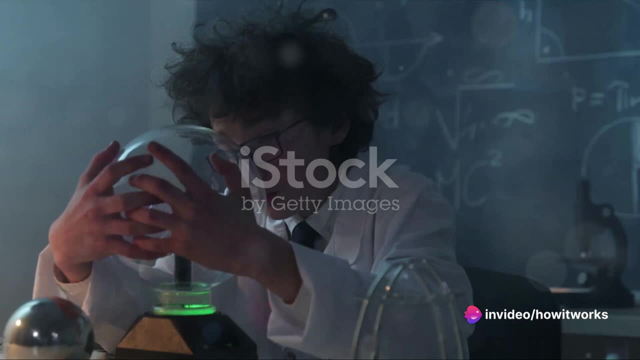 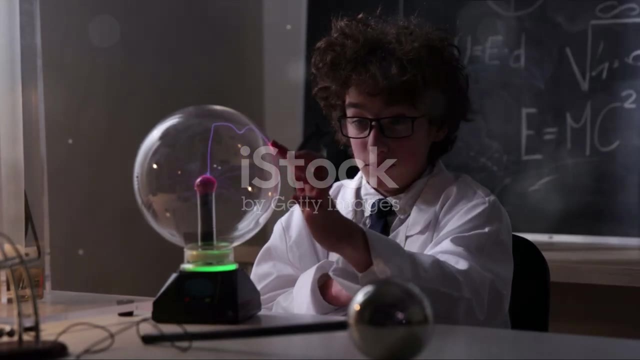 apple that rots away after a few weeks. a proton, as far as we know, seems to last forever. However, in the world of particle physics, there's a theory that suggests a different story. It's the idea of proton decay. Now, don't let that term scare you. It's not as complicated as it sounds. Think of it. 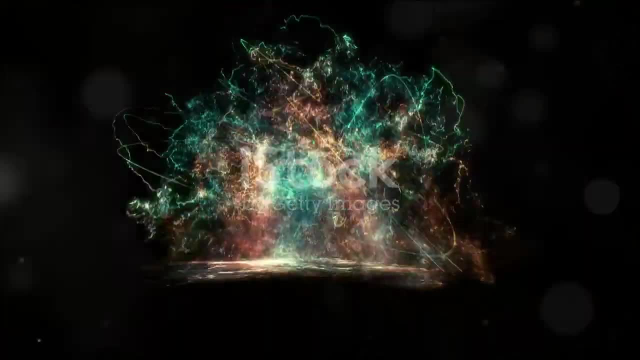 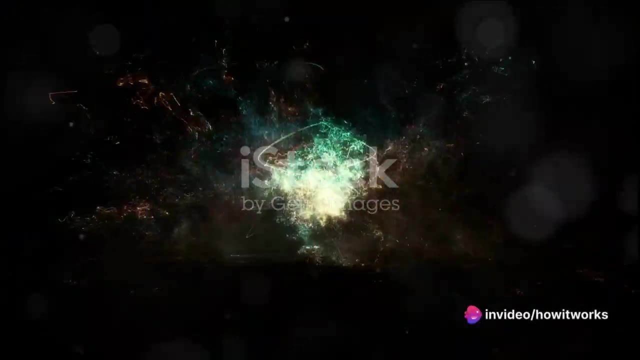 as our proton apple, gradually rotting away. But instead of a few weeks, this decay process takes an incredibly long time, far beyond our usual understanding of time. We're talking about a timeframe that is so vast it's almost impossible to wrap our heads around it. Imagine a clock. 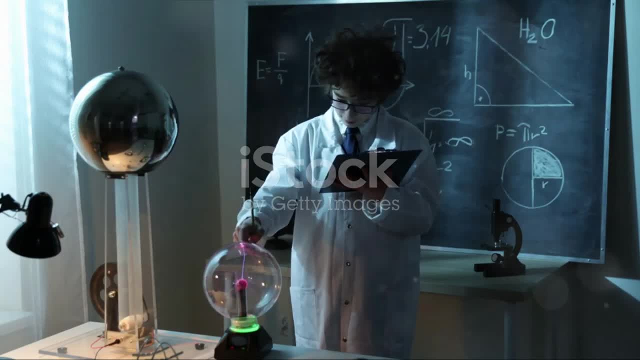 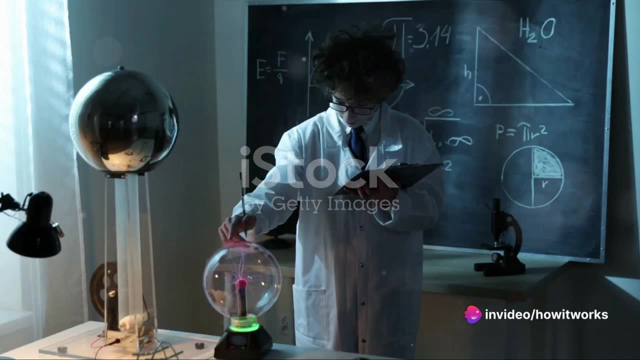 but this clock doesn't tick every second or every minute, or even every second Every year. No, this clock ticks once every ten to the thirty-fourth years. That's a one, followed by thirty-four zeros, A timeframe so long, it's practically eternity in human terms. 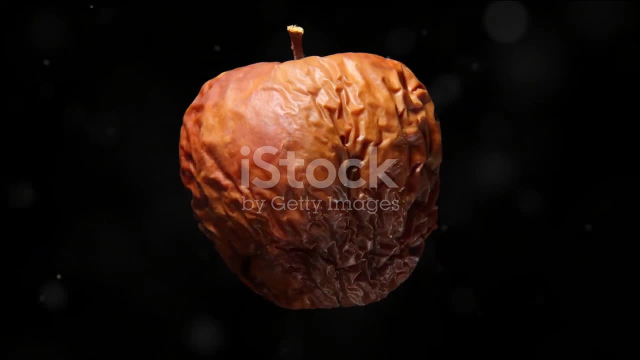 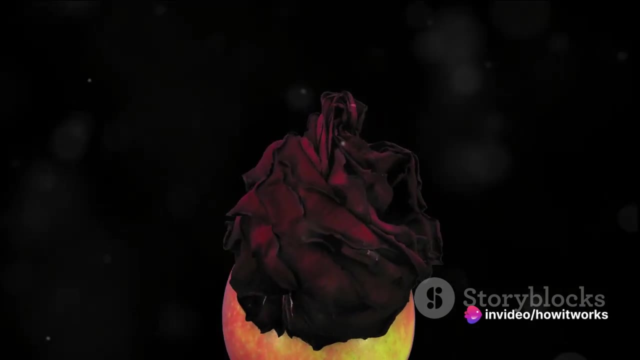 So what does this mean for our proton apple? Well, it means that if proton decay is real, then our proton apple, like a real apple, can indeed rot, But it doesn't happen overnight. It's a process that takes place over an unimaginably long period of time. Yes, our apple. 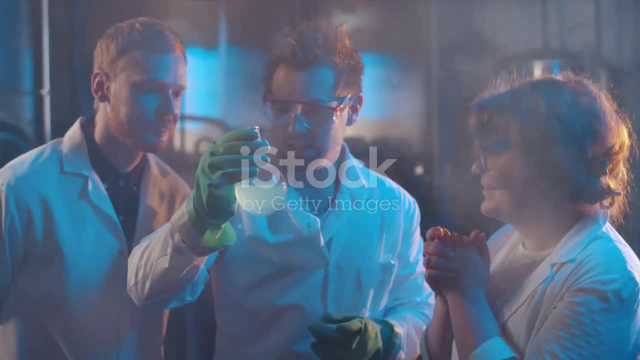 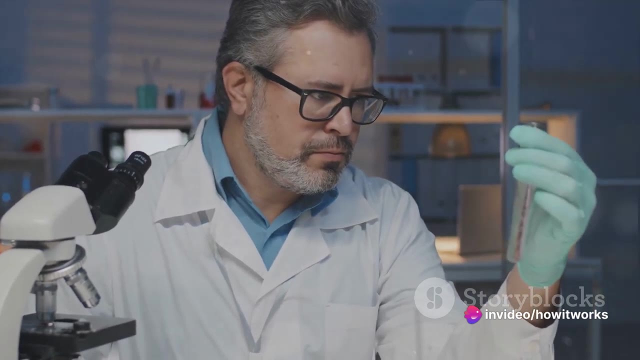 can indeed rot, but over a timeframe that is difficult to comprehend. This is where our story begins, So stay with us as we delve deeper into this fascinating concept in the next scenes. Trust me, it's going to be a mind-blowing journey To understand why and how a proton might decay. 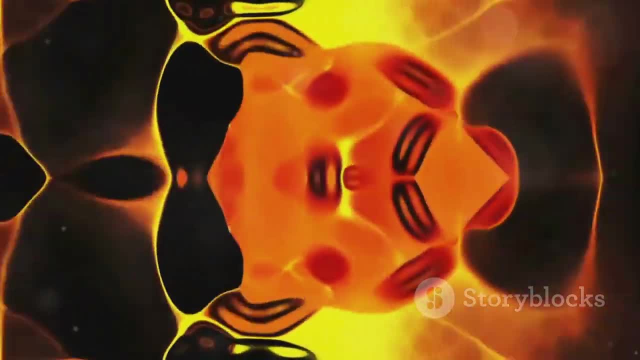 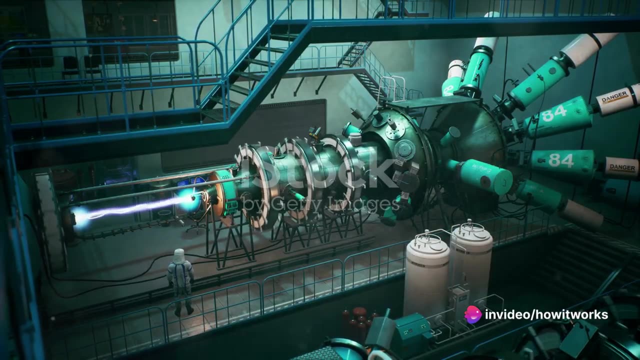 we need to dive into the realm of Grand Unified Theories or GUTS. Grand Unified Theories, or GUTS for short, are a sort of mega-theory in the world of physics. These theories aim to unify or bring together the three fundamental forces of nature. 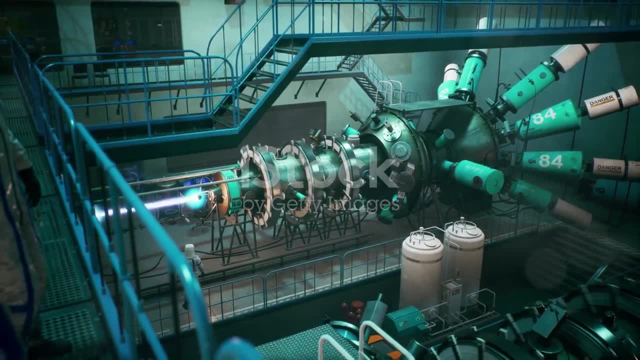 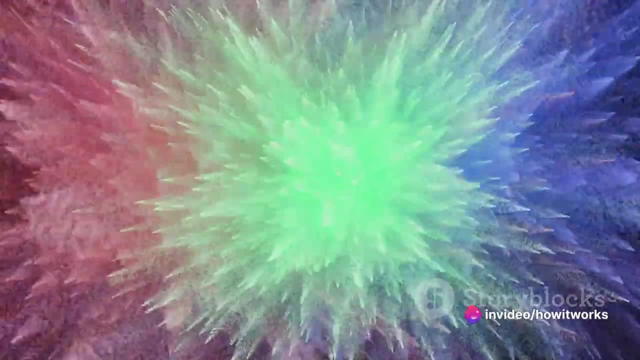 the strong nuclear force, the weak nuclear force and electromagnetism under one umbrella. Imagine these three forces as three different languages. Each has its own set of rules and vocabulary, making them distinct from one another. Now, GUTS are like a universal translator. 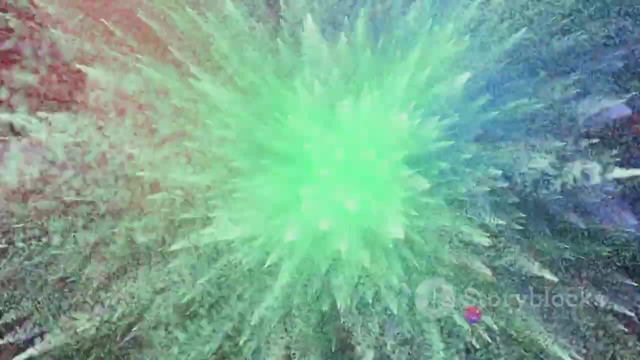 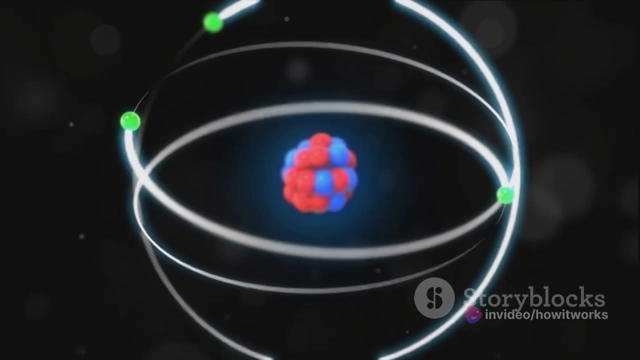 capable of interpreting all three languages and highlighting their commonalities. So where does proton decay fit into all of this? Well, GUTS predict that protons, the stable particles that make up the atomic nucleus, can actually decay. This is a radical concept, as our current 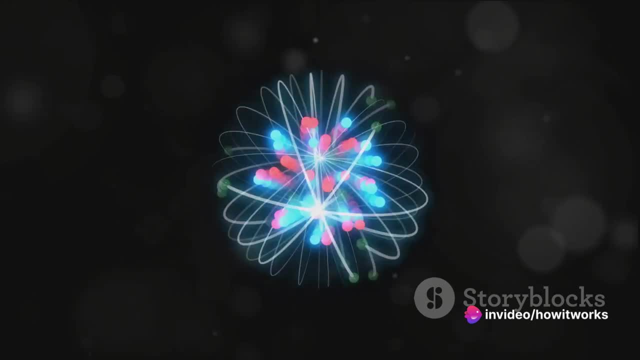 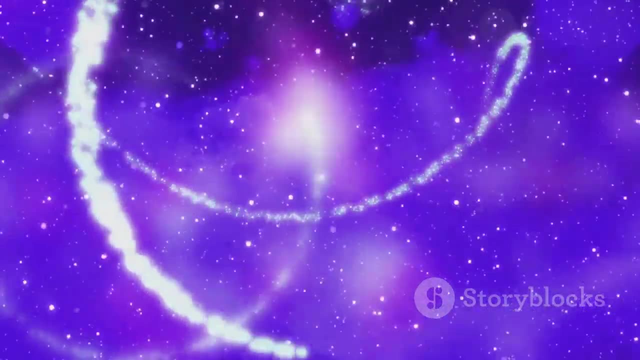 understanding of physics deems protons to be virtually indestructible. So let's get started. But GUTS suggest otherwise. They propose that, given enough time- and we're talking about a timescale so vast it's hard to comprehend- a proton could decay into a positron and a neutral. 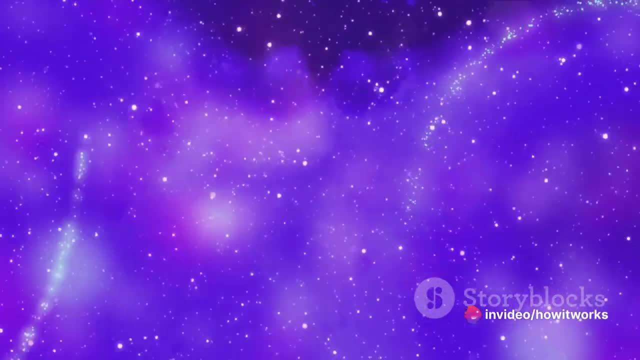 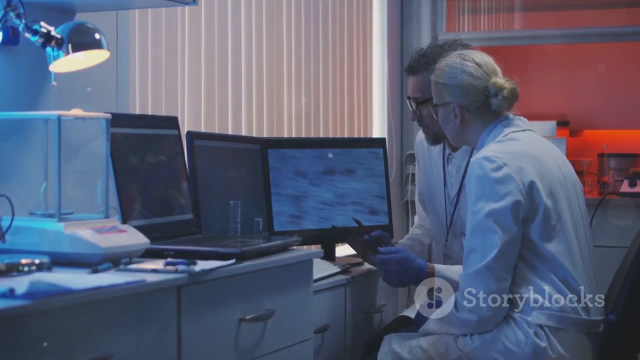 pion. This theoretical decay is a direct consequence of the unification of forces under GUTs. The significance of proton decay prediction goes beyond just shaking up our understanding of proton stability. It's a crucial test for the validity of GUTS. 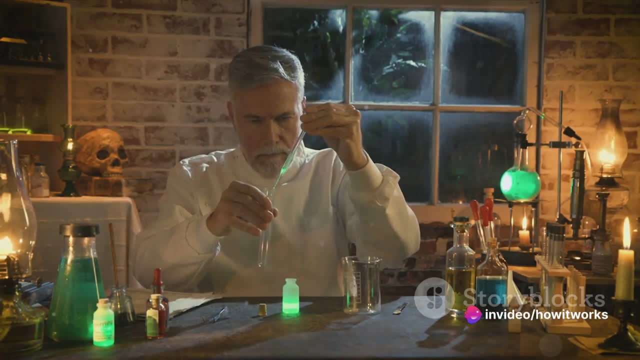 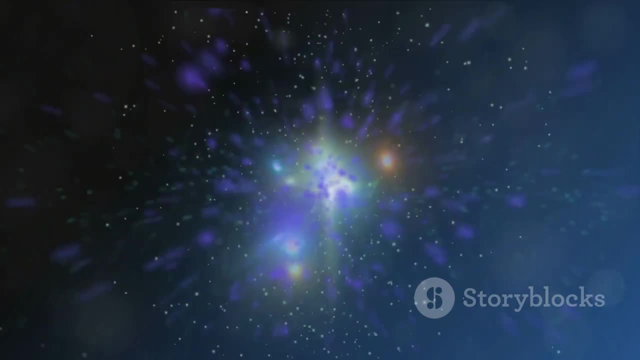 If we observe a proton decay, it would be a monumental piece of evidence supporting these grand theories. It would show us that our universal translator is on the right track. On the other hand, if we never observe a proton decay, it would suggest that our GUTS might. 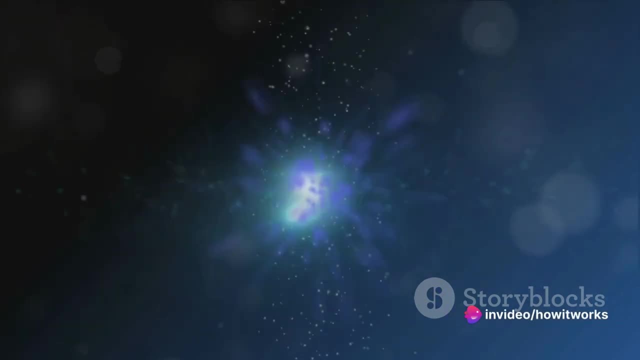 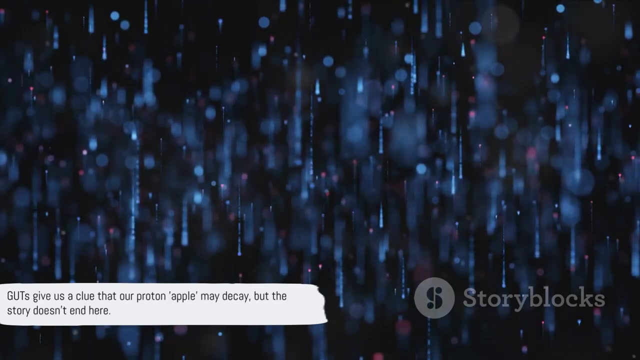 need some tweaking, It would be back to the drawing board to refine our theories and seek new ways to understand the fundamental forces of nature. GUTS give us a clue that our proton apple may decay, But the story doesn't end here. Enter the world of supersymmetry. 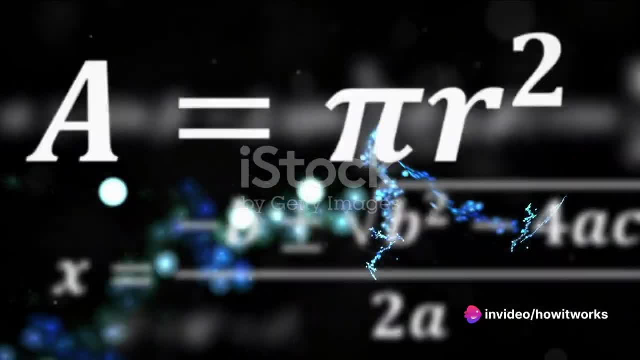 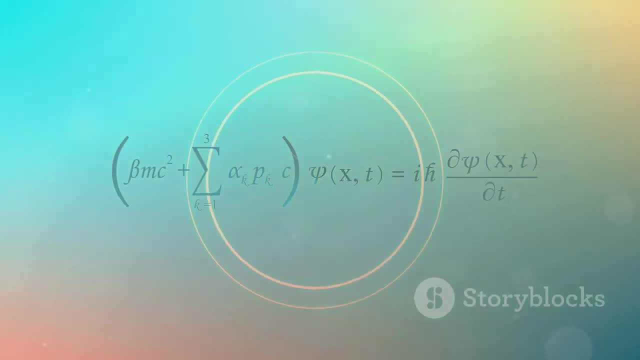 another fascinating concept from the realm of physics. To put it simply, supersymmetry is a proposed theory that suggests every particle we know has a superpartner with slightly different characteristics. Imagine having a twin from another universe, identical in most ways but with 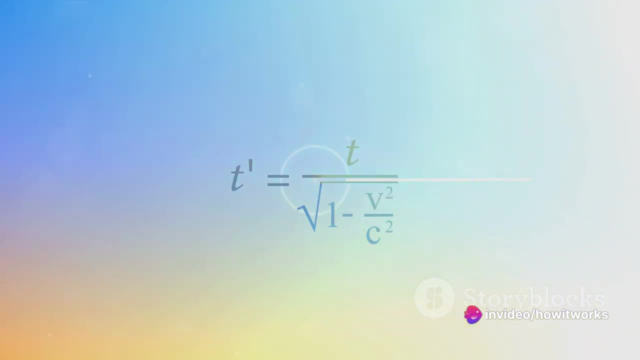 just a few tweaks to make things interesting. In the world of particles, these tweaks could be differences in spin, charge or other quantum properties. This is the essence of supersymmetry, often shortened to SUSY. Now you might be wondering: what does this have to do with proton? 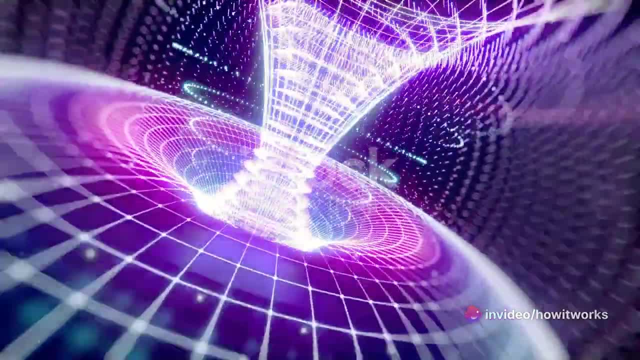 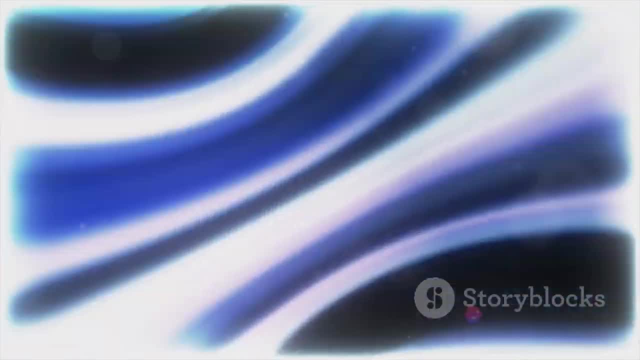 decay? Well, the answer to that lies in the heart of grand unified theories, or GUTS In the simplest terms, GUTS aim to unify all fundamental forces of nature into a single theoretical framework. That's where supersymmetry steps in, offering a potential bridge to connect. 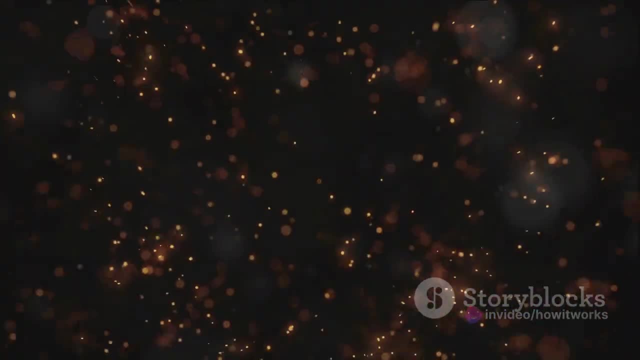 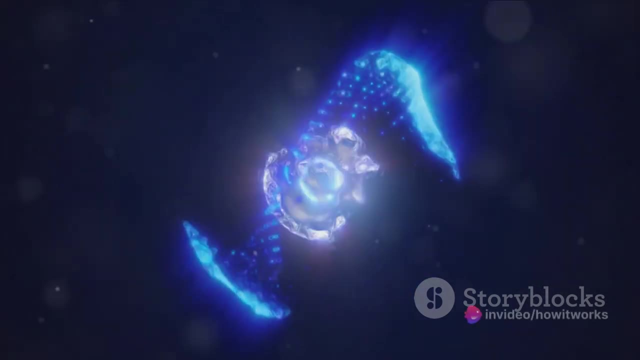 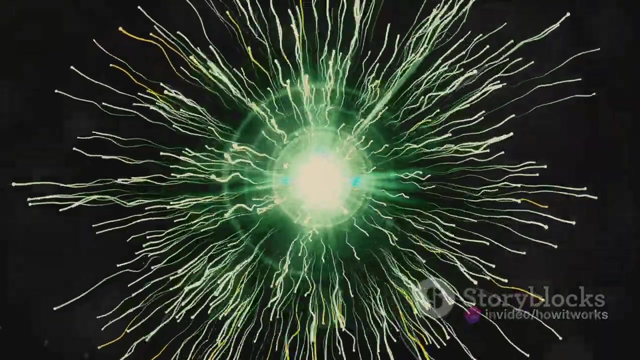 these forces. Supersymmetry predicts the existence of superheavy particles called sparticles, which can mediate proton decay. These particles can potentially interact with protons, triggering their decay into more fundamental particles. This interaction is what could potentially lead to the elusive proton decay we've been discussing. 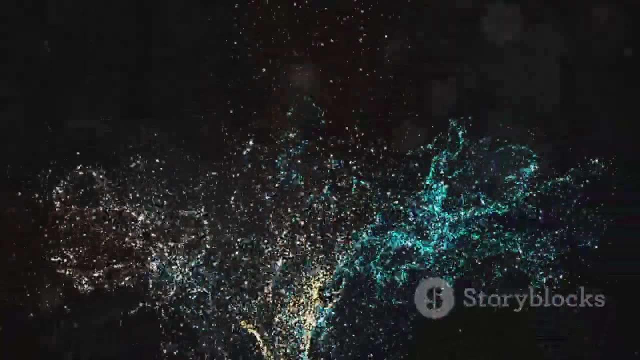 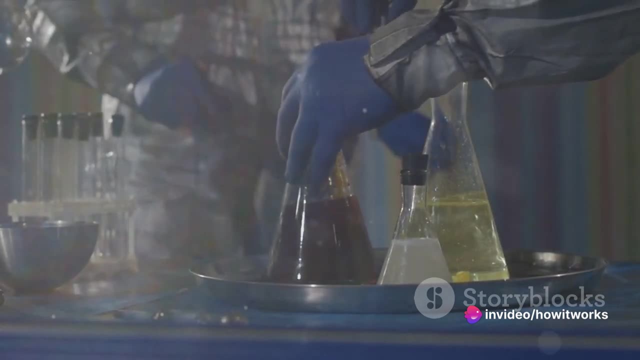 Here's the catch: The predicted rate of proton decay in supersymmetric theories is much longer than the age of the universe. That's right. according to SUSY, protons should be incredibly stable, with a decay time longer than the universe has existed. This poses a challenge for physicists. 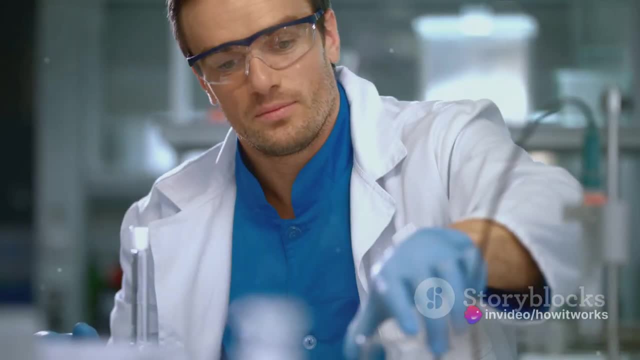 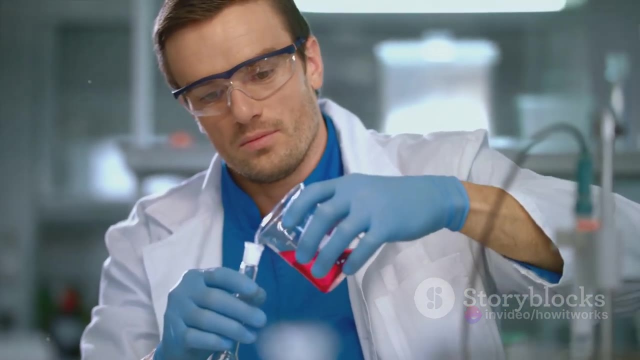 as it's something we have yet to observe experimentally. Despite the difficulties, the search for proton decay continues, with physicists worldwide hoping to catch a glimpse of this rare event. In the grand scheme of things, supersymmetry not only provides a possible 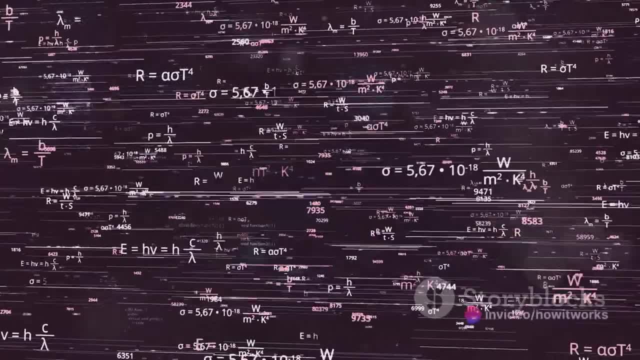 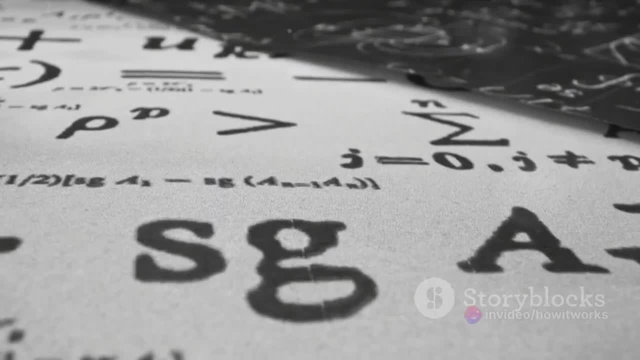 explanation for proton decay, but also brings us a step closer to unifying the fundamental forces of nature. It's a concept that pushes the boundaries of our understanding, adding a new dimension to the way we perceive the universe. Supersymmetry adds another layer of complexity.